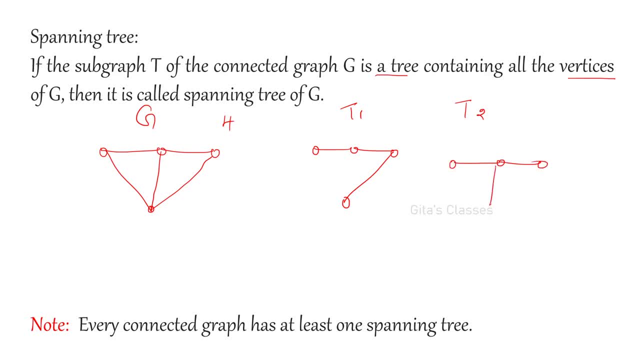 and you can have like this also. so, so, so, so, so. So it must have all the four vertices and it can have maximum tree means it can have only n minus 1 edges, n vertices and n minus 1 edges only. So this is T1 and T2 are examples of spanning trees. 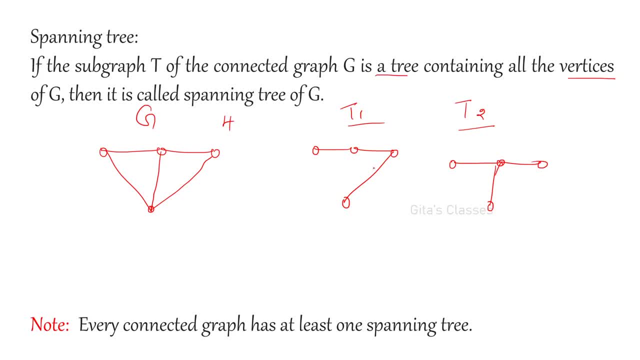 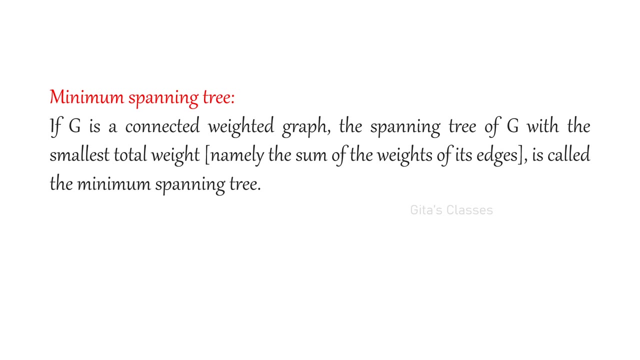 And every connected graph and it is not unique. You can have your own spanning graph, Only it should satisfy the conditions. So every connected graph has at least one spanning tree And minimum spanning tree if we find the minimum spanning tree for weighted graphs. 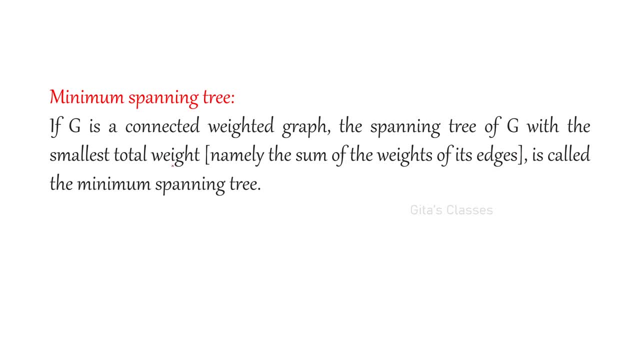 connected weighted graphs. the spanning tree G with smallest total weight- that is, the sum of the weights of all its edges. if you add it should be minimum- is called the minimum spanning tree And we have some algorithms for finding the spanning tree. 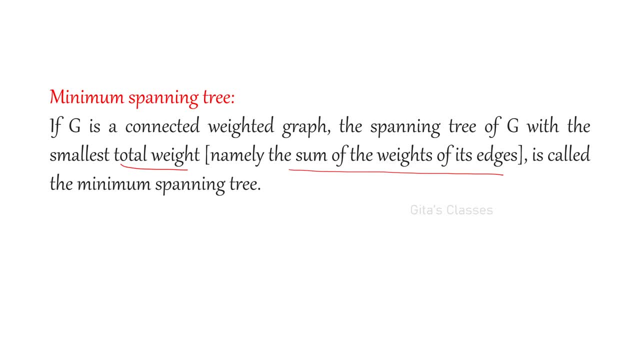 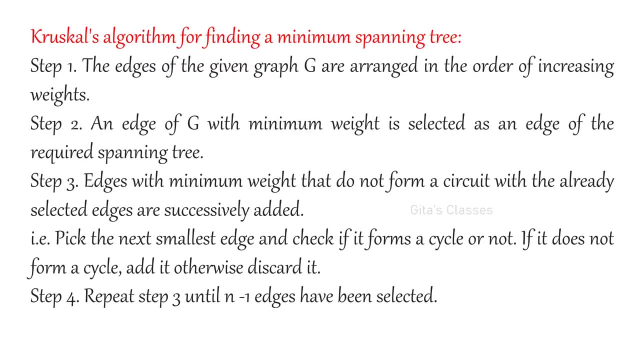 It is very, very important topic. So we have two algorithms: One is Kruskal's algorithm And Prim's algorithm. Let us see what is Kruskal's algorithm for finding the minimum spanning tree. So first step is you write all the weights, all the edges of the, the edges of the given. 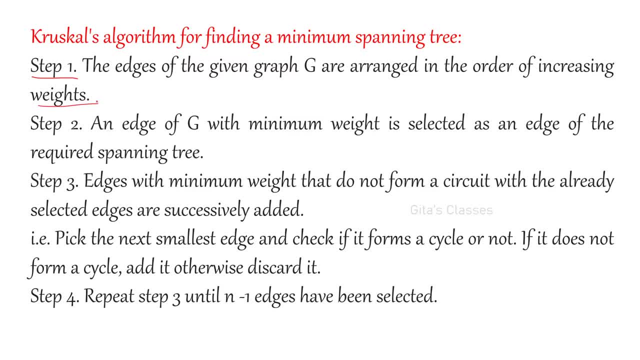 graph G are arranged in the order of increasing weights. Okay, For all the edges will have some weights. Weight means some number will be assigned. Okay, For example, it may be, if you consider all the places: Okay, All the cities as a, as a. 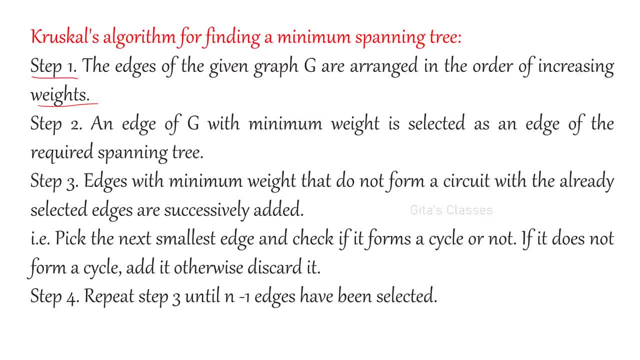 As vertices and the distance between the cities. So if you want to find out the travel minimum, travel distance, like that, So it is an application Okay. So if you want to find out the minimum spanning tree, it is equivalent to the finding the. 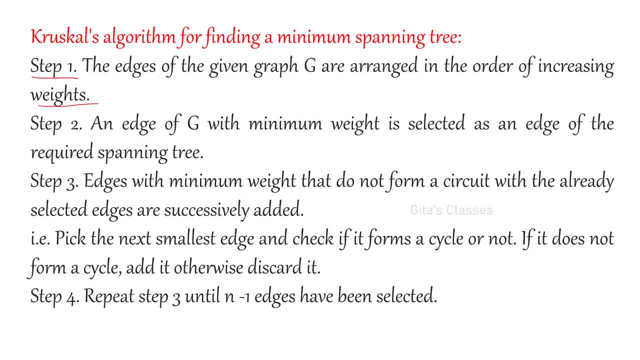 minimum spanning tree. If you want to find out the minimum distance between to be travel between the cities, then it is equivalent to: in graph theory, we can find out the minimum spanning tree. Okay, So the edges of the given graph G are arranged in the increasing. 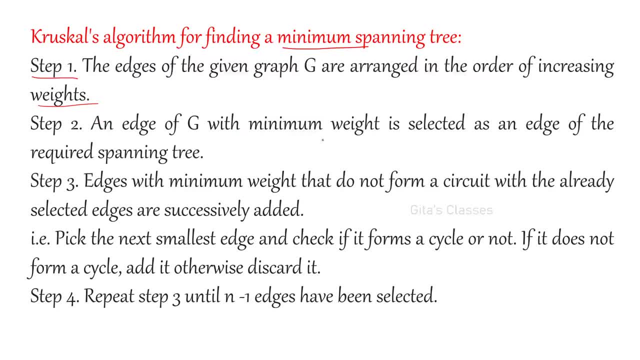 Order of weights. then an edge G with minimum weight is selected as an edge of the required spanning tree, and the edges with minimum weight that do not form a circuit with already selected edges are successively added. Then pick the next, that is, pick the next smallest yet. 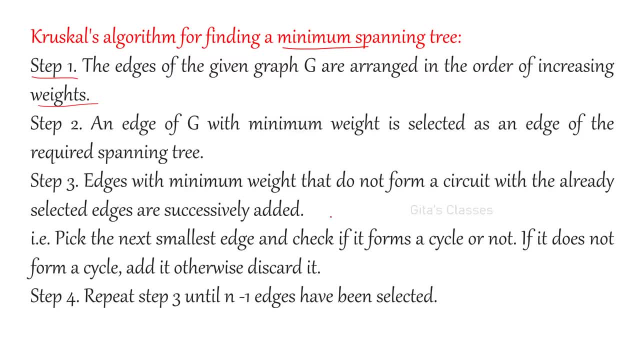 And if it is forming a cycle, don't add, otherwise you add. Okay, So it forms a cycle or not. If it does not form a cycle, add it, Otherwise discard it. Okay, Then step three is done. repeated until n minus one edge has been has been added. 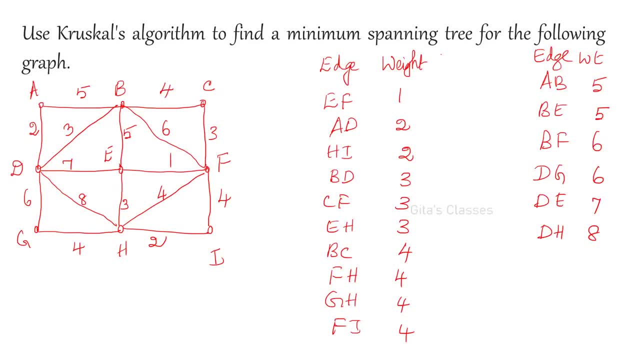 Okay, So let us see. you will understand one example. then you will understand this clearly. Use Kruskal's algorithm to find the minimum spanning tree for the following graph. This is the graph G, Right? This is the graph G. 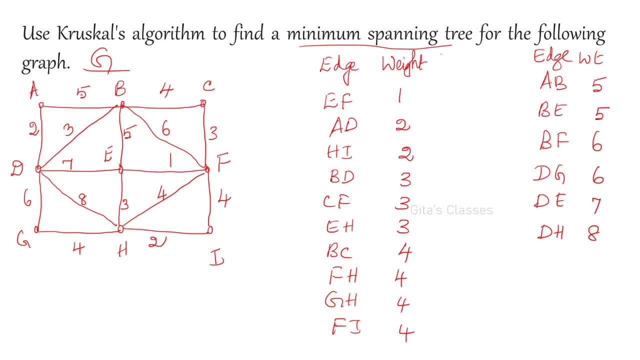 And from. you have to order, you have to select. see so many numbers are there: 5, 4,, 2, 3, 5, 6, 3 and so on. So search for the minimum value. 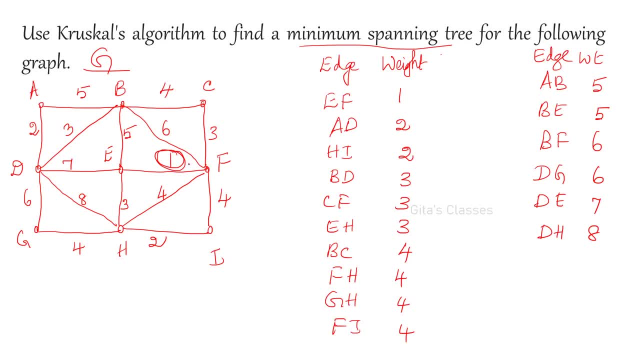 What is this? minimum value is one which edge is having one EF, So you write EF first. Okay, Then we have two. AD is having two, So AD is equal to two. HI is also having two. You can interchange. you can write first HI two and AD two, also, no problem. 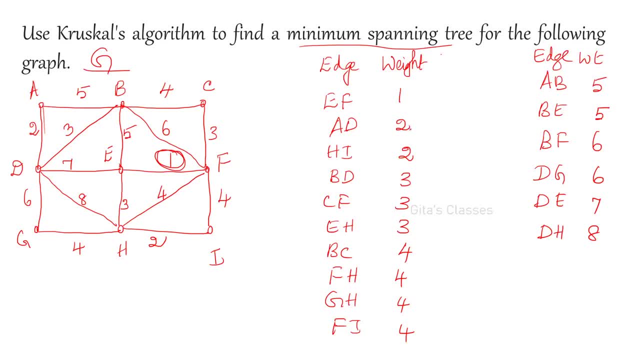 And always remember the minimum. the spanning tree need not be unique. Okay, Sometimes you will add this edge or that edge, no problem. AD and HI, Okay, Then B. BD then is three, Okay, So three. we have BD, CF, EF and so on. 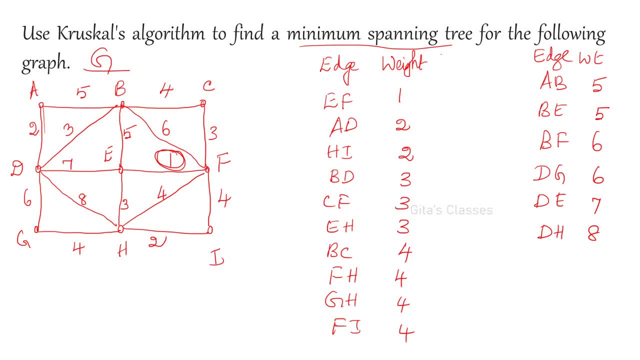 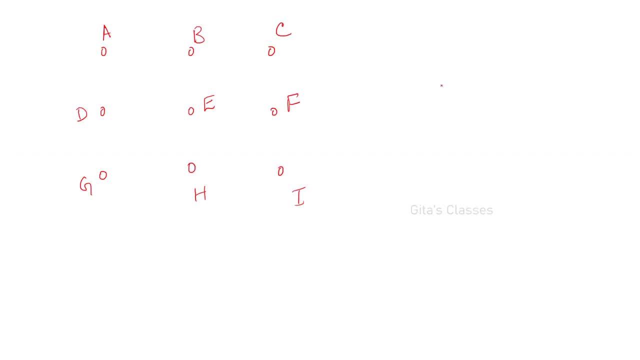 So we have formed, arranged in ascending order. Then you should keep on adding. First let us add EF. Okay, EF, this is the first one. So I have drawn here. So edges are available. I will keep on adding the edges. 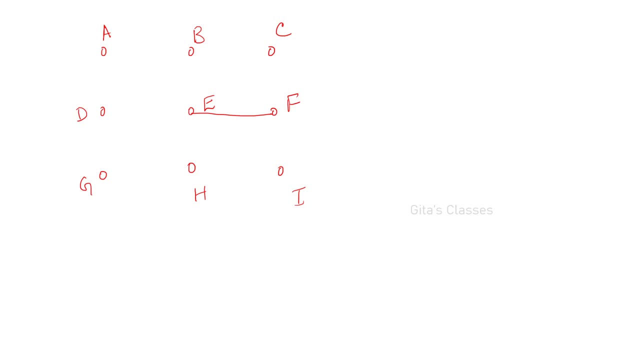 First you, because the spanning tree must contain all the vertices, right? So you write all the vertices first. That is the first step. You write all the vertices for drawing the graph. you write all the vertices, Then you keep on adding the edges without forming the cycle. 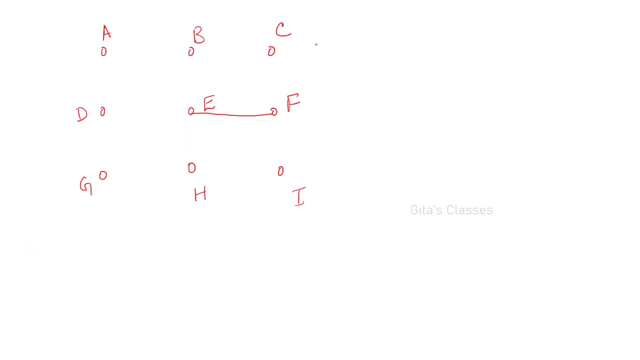 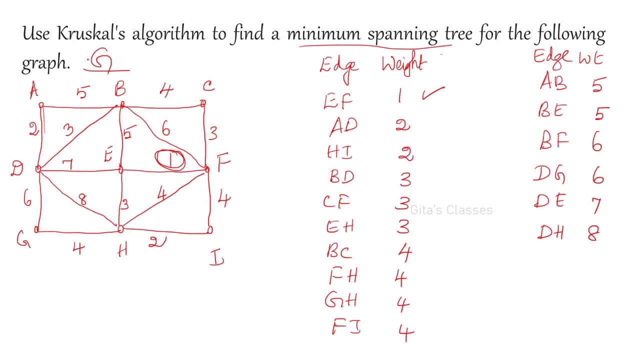 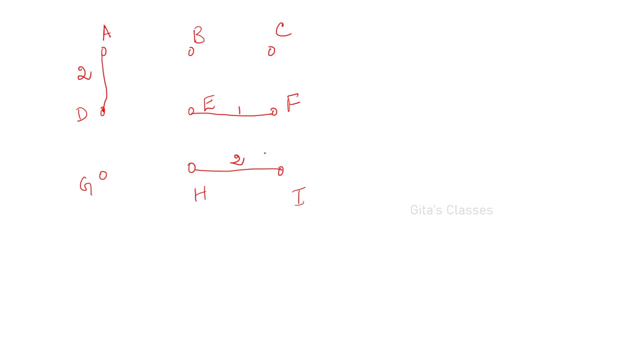 That is the main point. AD is equal to two. You write the weight also here, AD you have. you have to add AD. Then HI is two, HI is two. Before drawing you find out whether it is forming a cycle or not. 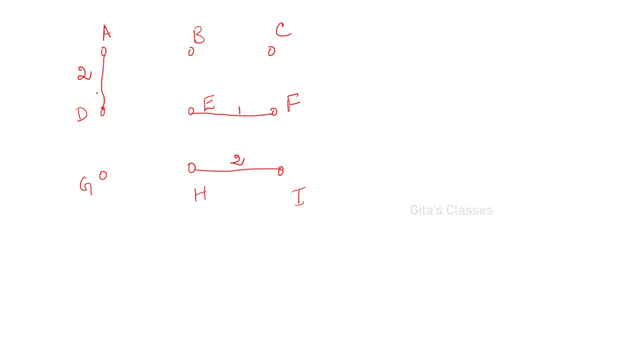 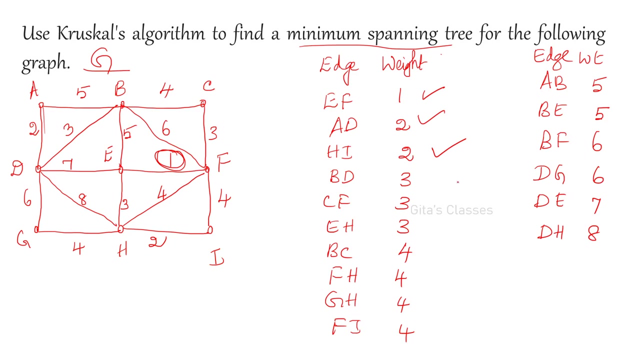 If it forms a cycle, then don't add. Okay Then. so this is added. this is added. Next: BD is three BD. will it form a cycle? No, BD three. Yes, we can add. We have added: BD is three. 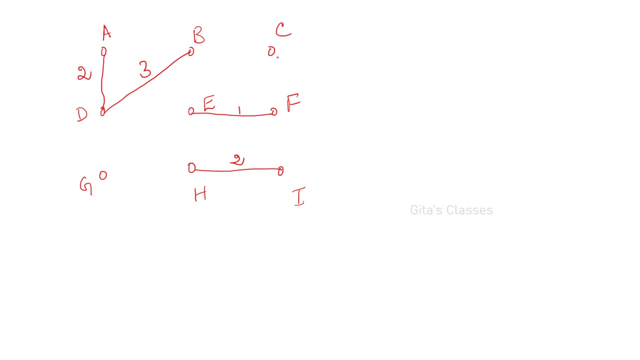 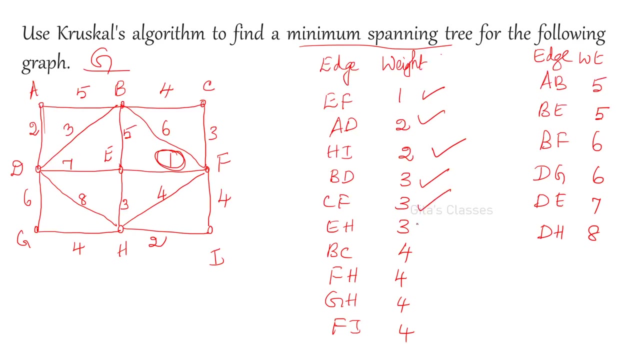 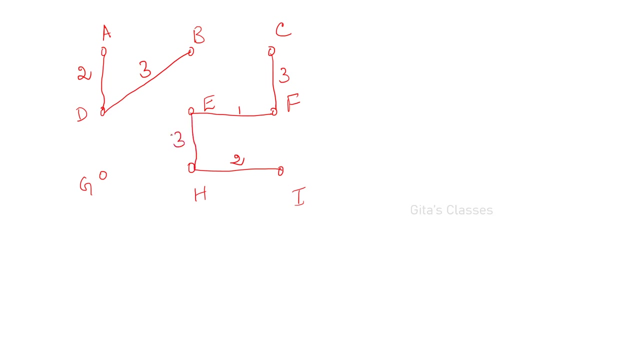 Next, what is CF? is three CF three? Yes, it is not forming a cycle, we can add, So CF three is added. What about EH three? EH, Yeah, even this is not forming a cycle, So EH three is added. 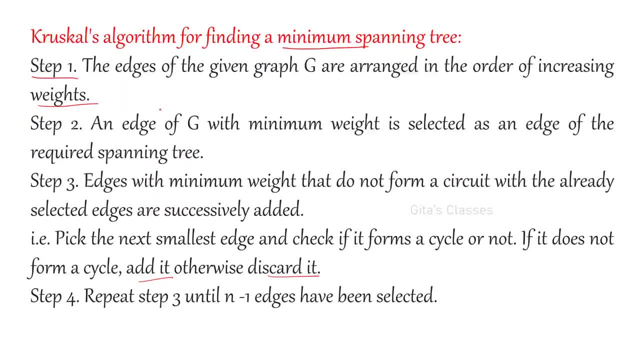 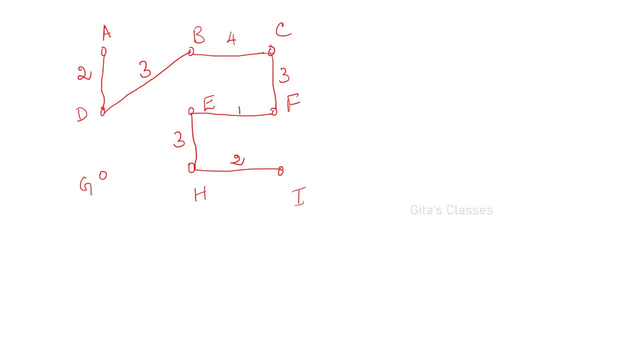 Then BC is equal to four, BC four. Yes, even if you draw this, it will not form a cycle, So you can add: Okay, BC is four. Then next is BC four is added. What about FH four? 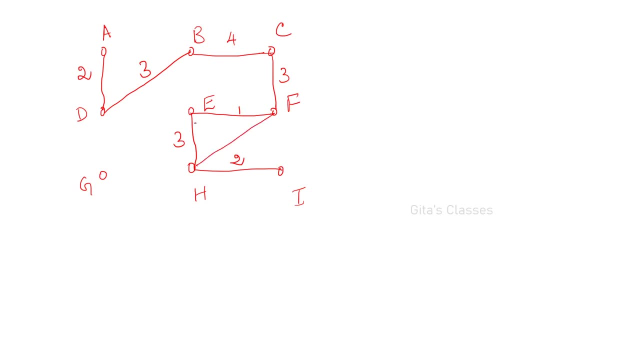 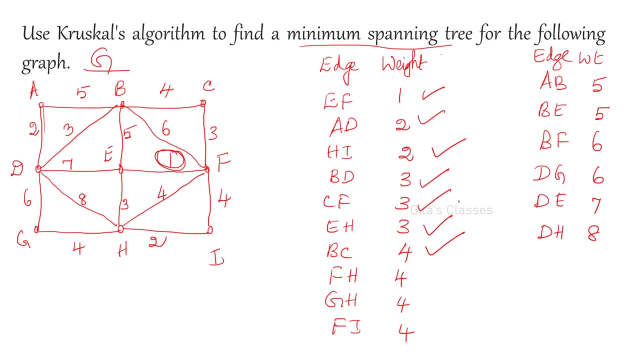 FH four. if I draw this, it is forming a cycle. This will form a cycle. no, So don't add this. FH is not added. Okay, FH should not be added. What about GH then? GH, GH is four. 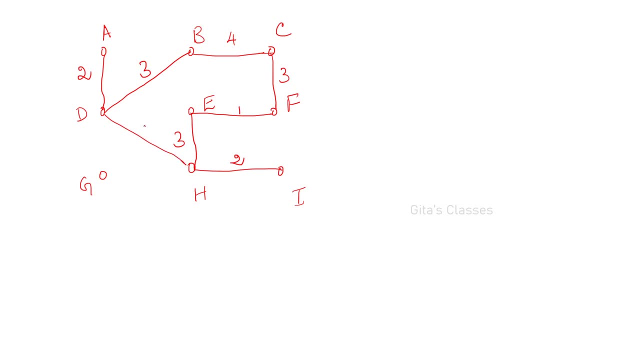 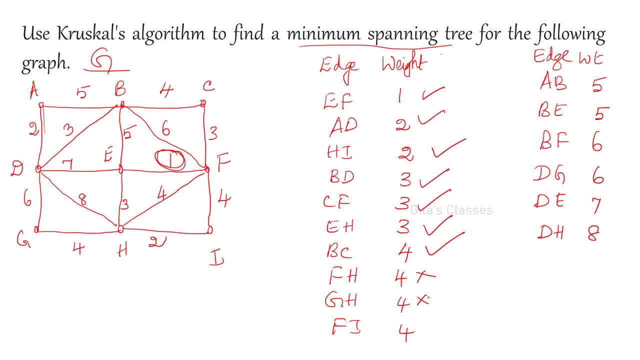 Even GH will form a cycle, So don't add. If you add this, it is forming a cycle, So don't add GH. So GH is not added. What about FI GH? if I add, will it form a cycle? 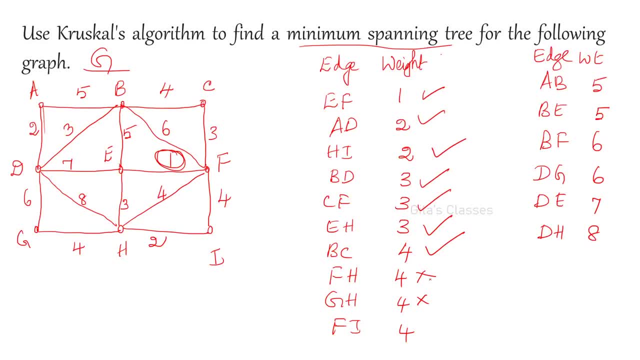 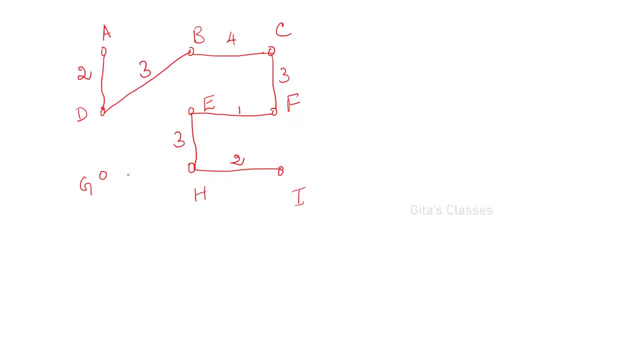 GH. sorry, wait, wait, GH can be added. FH cannot be added. GH has to be added. sorry, GH is four here. I saw with the D, So this is four. Okay, GH is four can be added because it does not form a cycle. 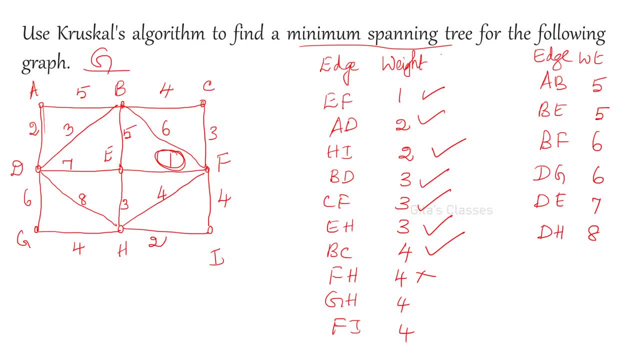 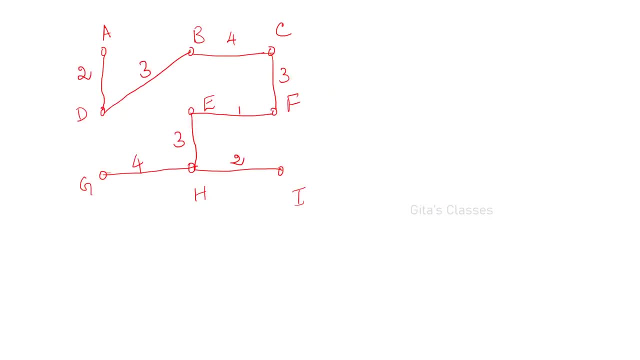 I checked with D. That's why It was a cycle. So GH is added. What about FI? FI will form a cycle. So don't add. FI cannot be added. Then you can check with the remaining. also, AB will form a cycle. 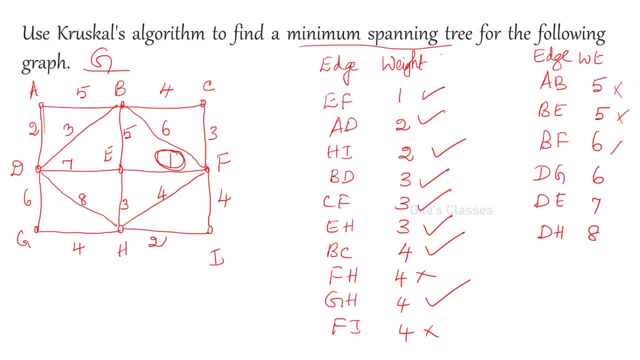 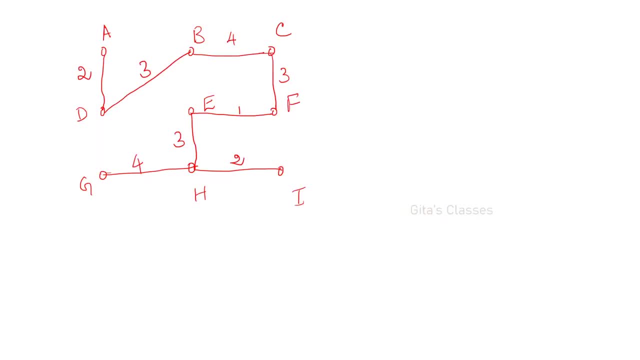 All the remaining you cannot add, So these need not be added. You can check with all the other vertices. If you add all the edges, they will form a cycle. So this is our And we got here. how many? What Vertices are there? 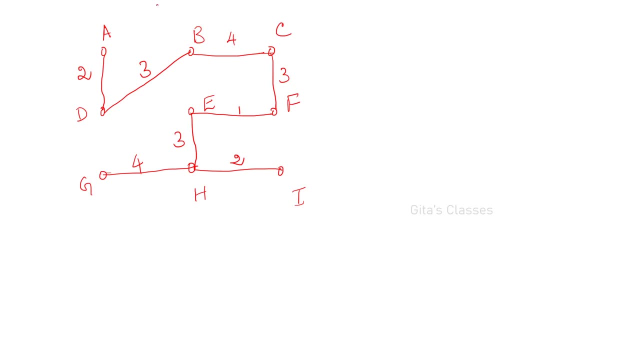 Nine vertices are there? No, So eight edges you should get. So one, two, three, four, five, six, seven, eight edges already we have formed. So we have formed the spanning tree. Okay, So this N is because N is equal to nine. 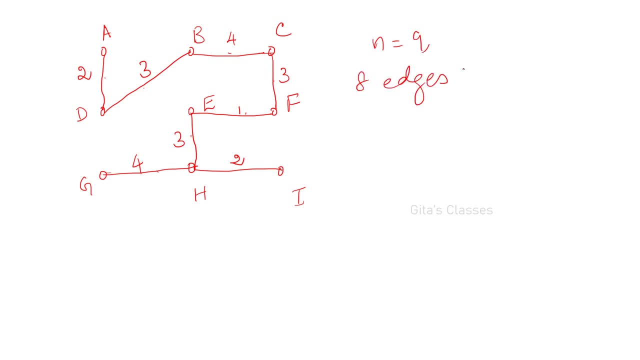 Only eight edges are allowed to form the tree Right. So eight edges are selected To form the tree And the minimum value- This is the minimum Spanning tree. So what is the minimum weight? As I have told you, if you want to find out the minimum distance in the real life example, 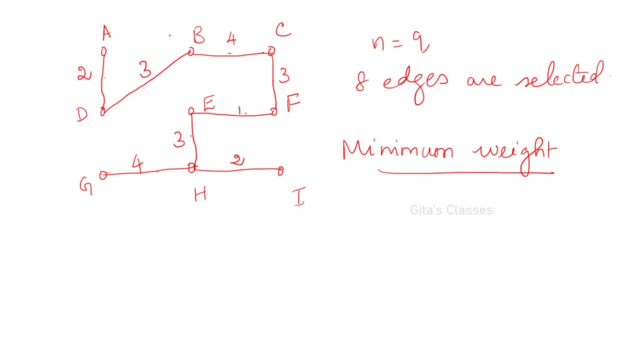 minimum distance between the cities. Okay, So minimum weight is the distances. Now some numbers are given, So if you, it can be used for the for finding the minimum distance also. So what is the minimum weight? You have to add all these numbers. 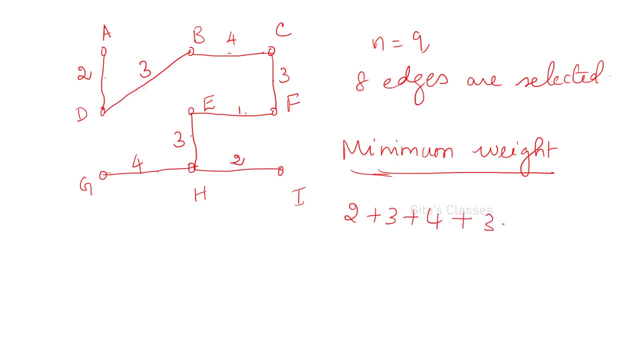 So two plus three plus four plus three Plus one plus three plus four plus two, That is five. nine then 13,, 13,, 17, plus six, 20.. I am getting 22 only here. 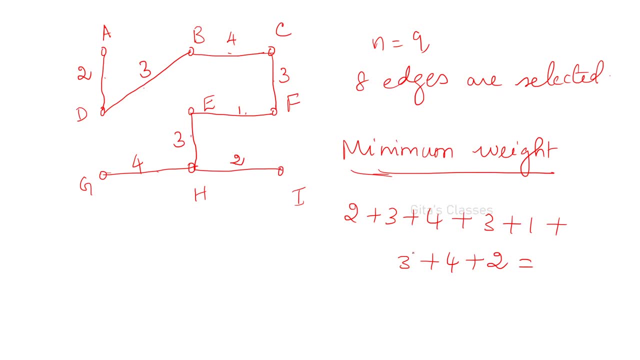 So two plus three, five, nine, 12,, 13,, 13,, 16.. Yes, 22. 22 is the weight. So minimum weight, Minimum weight is 22.. This is Kruskal's algorithm. Now we will see one more example in Prim's algorithm. 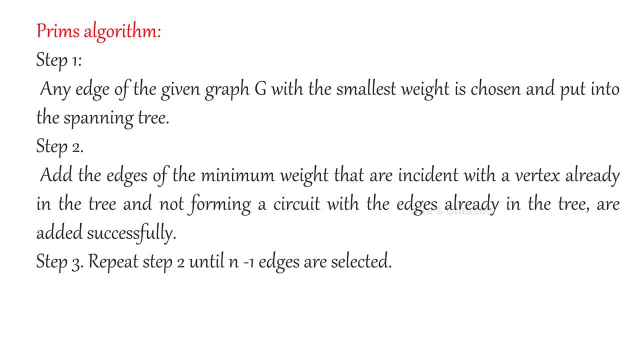 Prim's algorithm says that step one, any edge of the given graph G with smallest weight is chosen and put into the spanning tree. Okay, There in Kruskal's algorithm, we have arranged all the weights, We have written all the weights. 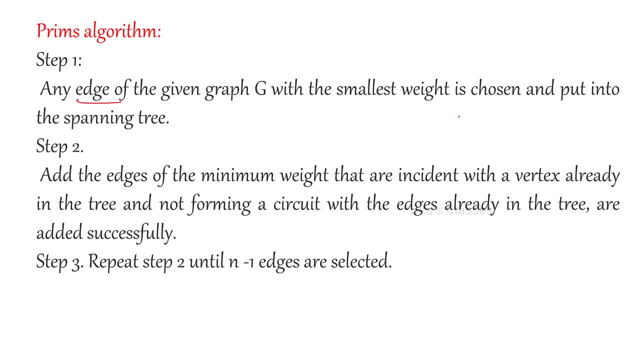 Here it is not like that. First you select one edge with minimum smallest weight, Okay. Then you find out which are all the edges. This is done with the smallest weight. Then you keep on adding them, Okay, Without forming a circuit. 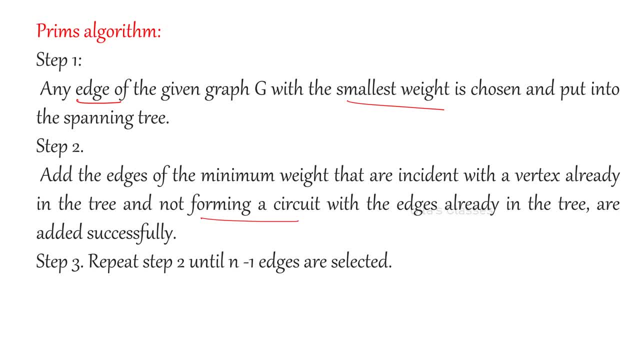 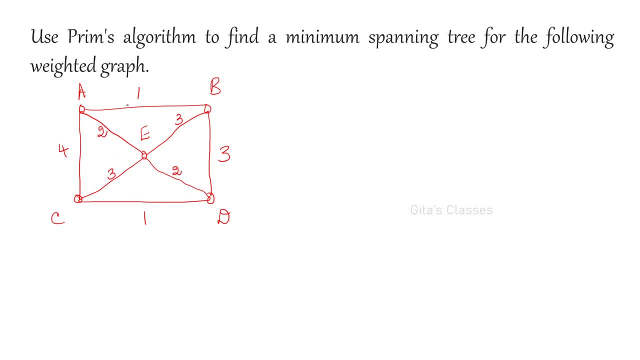 Repeat step two until n minus one edges are selected. Okay, So let us see one example Here: A, B, C, D, E. So which is the minimum weight? Either A, B or C D. I am going to select A B.